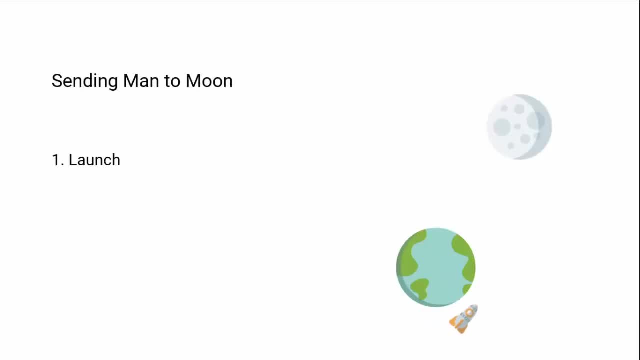 language that you like. Pseudocode is not just for beginners. It is a way of understanding a problem. Using it, you could quickly break down a bigger problem into smaller issues. This helps in bringing modularity and describing it on a high level. 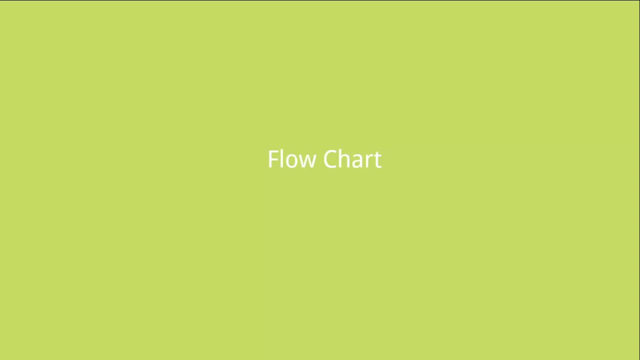 An algorithm can be visually represented using a flowchart. Being visual, it helps in understanding the logic quickly. Few basic symbols used for making flowcharts are: flowline, an arrow coming from one symbol and ending at another, symbol, which represents that the control passes. 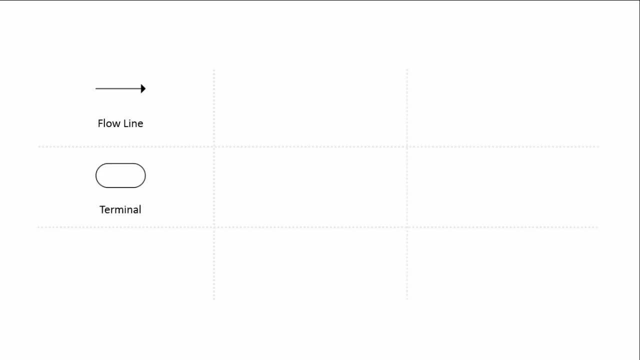 to the symbol. the arrow points to Terminal. denotes beginning or the end of the program Process. denotes that something is performed. Decision represents a decision. commonly it is a yes or no question, or true or false test. Input-output involves receiving data and displaying processed data Annotations. 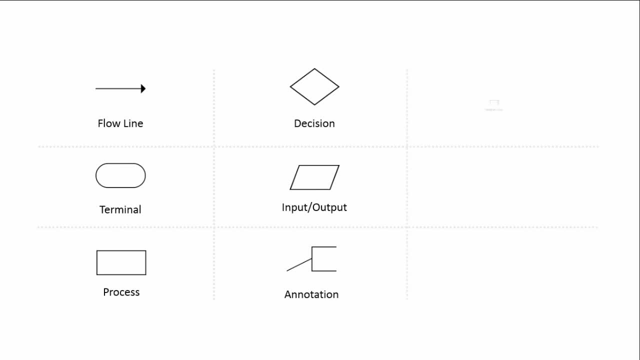 represents comments or remarks about flowchart Predefined process. these are used to show complex processing steps which may be detailed in a separate flowchart. Preparation shows operations for preparing value for a subsequent condition or decision. step Off-page connector used when there are multiple control flows which converge into 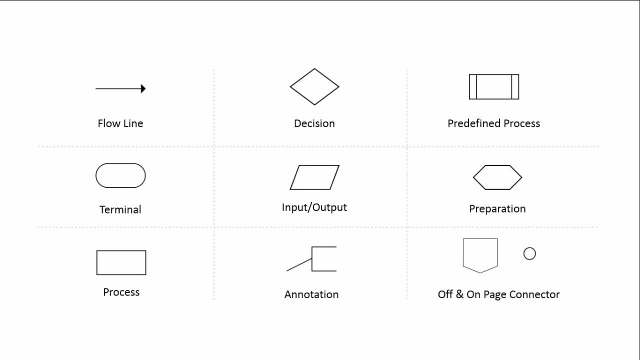 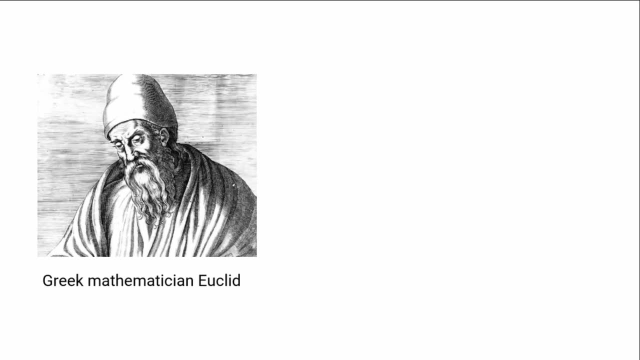 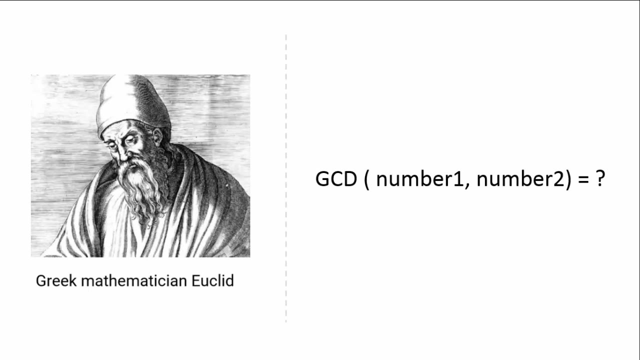 a single exit flow Off-page connector similar to the on-page connector, except it allows for placing a connector that connects to another page. We would further try to understand the flowchart by taking a problem for calculating the GCD of two digits using Euclid's algorithm. 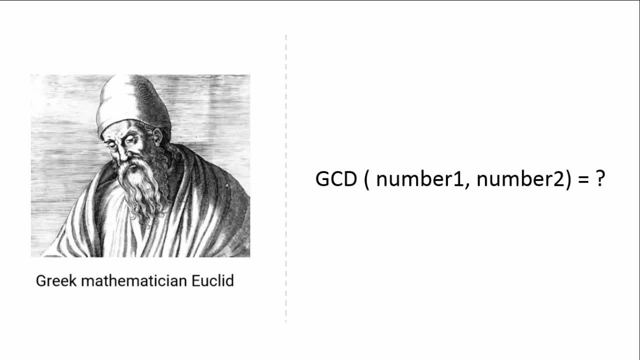 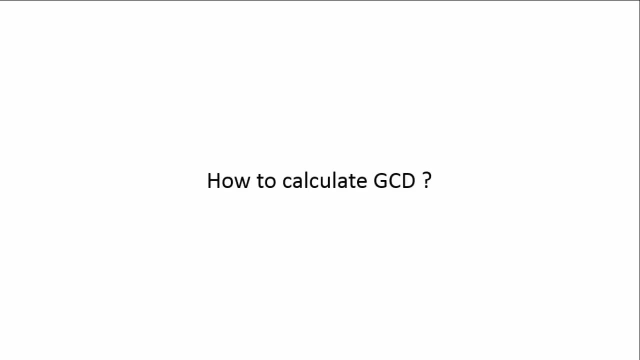 The most common divisor, also known as the GCD, of set of numbers is the largest positive integer number that divides all the other numbers in the set without any remainder. It is the biggest multiple of all the numbers in the set. If we take a specific example, 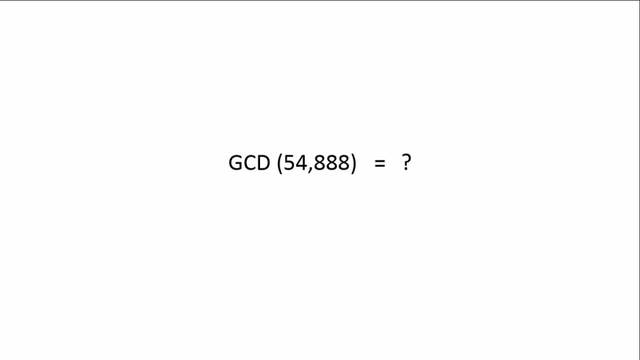 with two numbers, 54 and 888,. we know that the least number that could divide both these numbers is 2, but there could also be some other number which is greater than 2 which divides both 54 and 888.. The algorithm proceeds by taking smaller of the two numbers and dividing the larger. 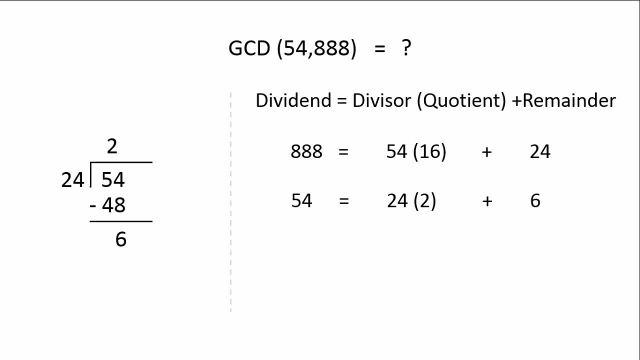 number by it. In our case, we will be dividing 888 by 54. So 16 times 54 will give you 864 and we get 24 as the remainder. We can write this down in the form of dividend equal to. 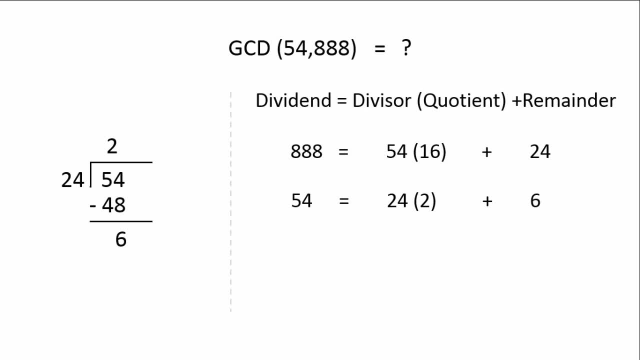 divisor multiplied by the quotient and adding the remainder. Now, as per the algorithm, we continue dividing the quotient by the remainder and we continue this till the remainder is 0.. As per the algorithm, once you get 0 as the remainder, then look up in the previous. 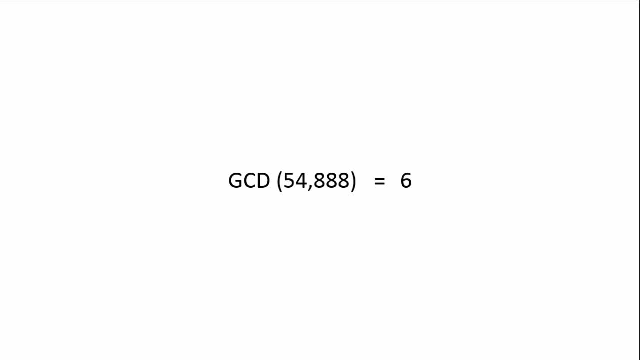 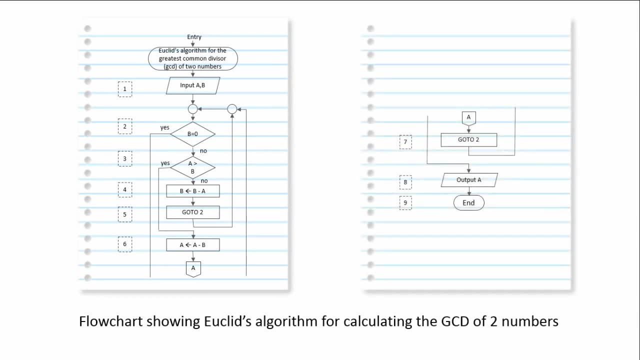 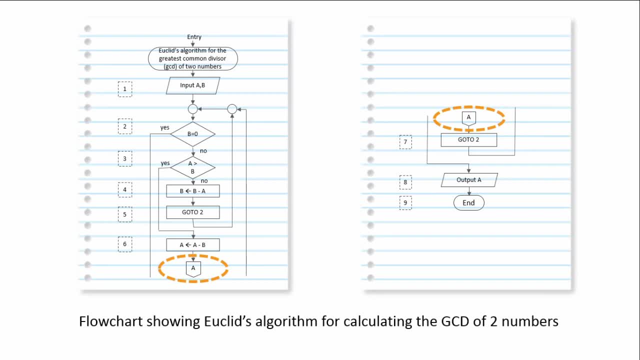 simple. Since the flowchart does not fit completely, we will just take the method, as it is quite simple. You can pause for a while and try to observe and understand the flowchart. We would break this down into smaller section and try to understand how this logic works. We will also do a dry run for calculating the GCD by substituting: 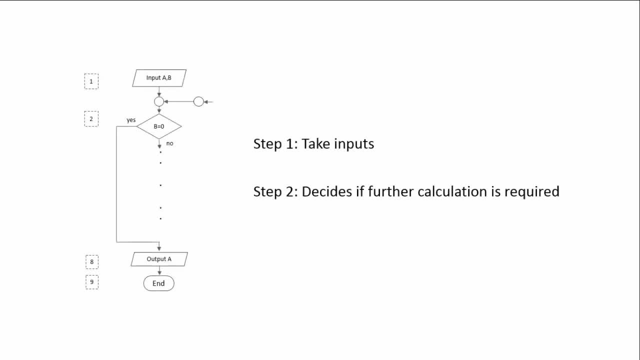 values in this logic. We will also do a dry run for calculating the GCD by substituting values. in this logic. The algorithm takes two numbers as input. Let us say that those two numbers are assigned to variable a and b. The flow continues, processing further instructions only if the value of b is not equal to zero. 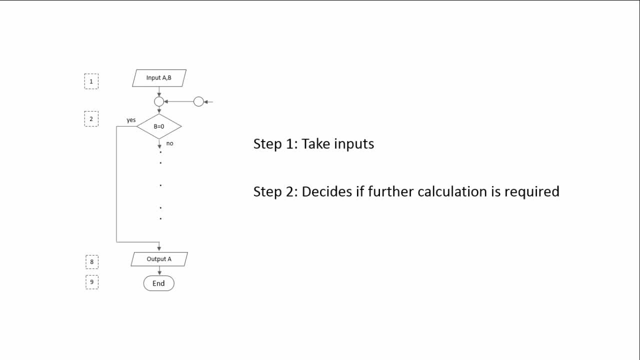 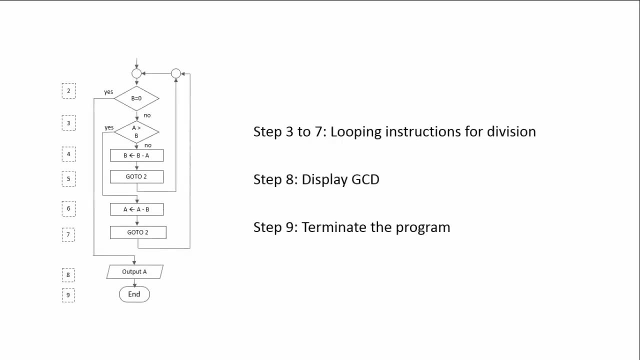 In step 2,. if the value of b is zero, then algorithm outputs the value assigned to variable a as the GCD. Step 3 to 7 are looping instructions, meaning that they will keep repeating until the condition of number b becoming equal to zero is satisfied. If value of a is greater than b. 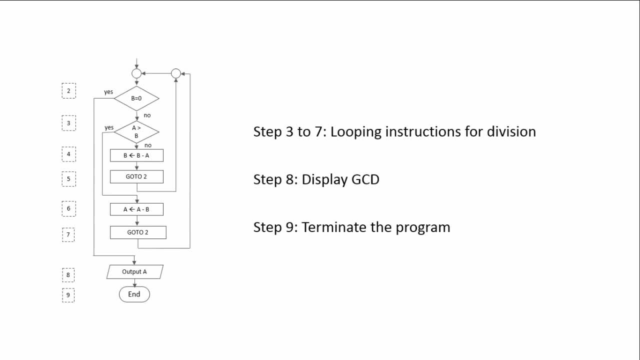 then we will subtract value of a from value of b and store the result in b. Alternatively, if the value of a is less than b, then we will subtract value of b from value of a and store the result in a. We are essentially performing division over here, similar to our previous.